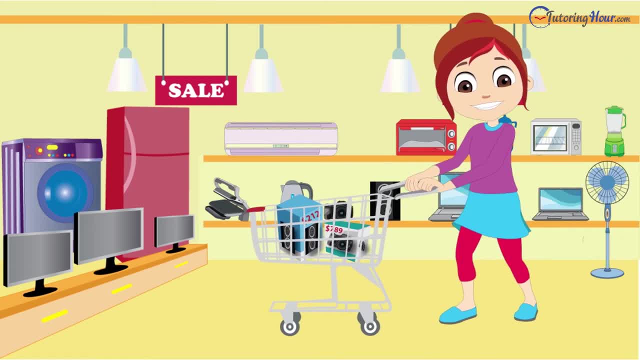 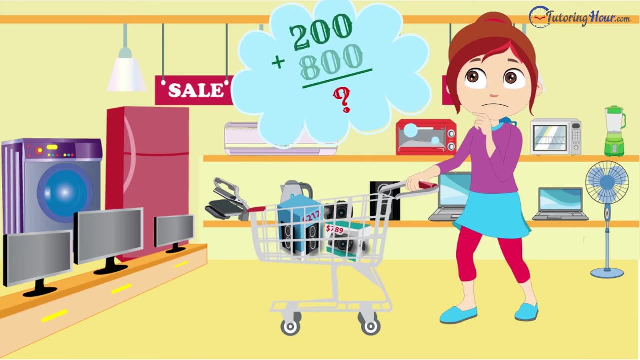 Let's think of this scenario: Debbie is buying electronic gadgets for $212 and $789. Adding these two amounts is taking her time. But what if the prices were $200 and $800? She could tell the total is $1,000 in the split second, right. 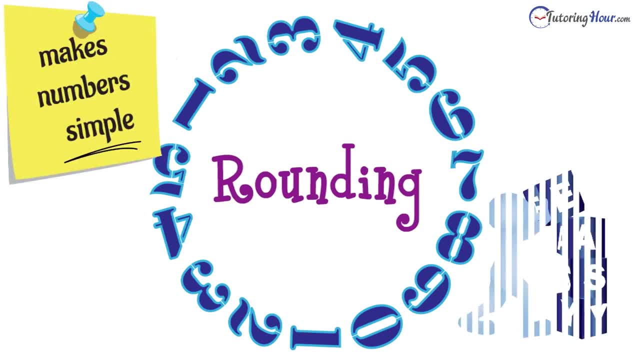 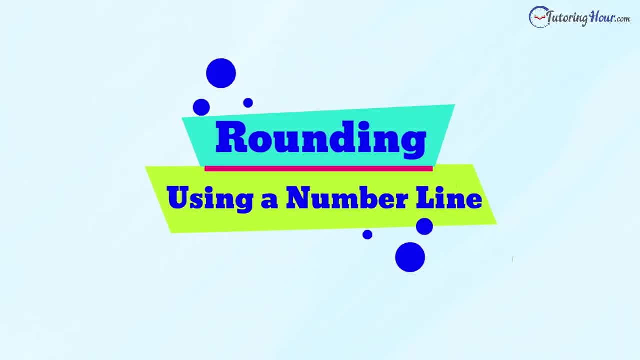 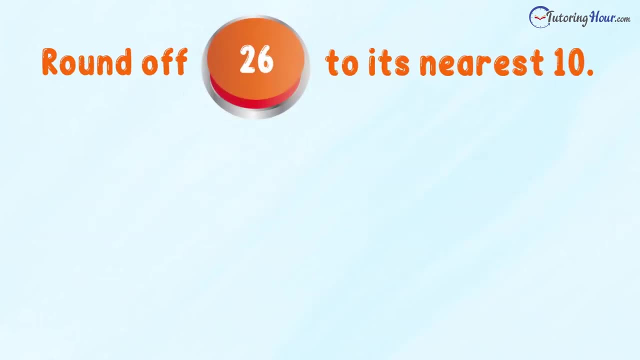 Rounding makes numbers simpler and easy to work with. Let's move on to the know-how of rounding using a number line and understand the underlying place value concept. We'll try rounding off the number 26 to its nearest ten. Let's do that by looking at the digit in the tens place. 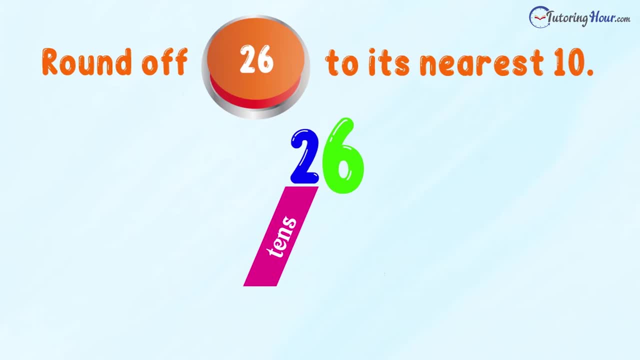 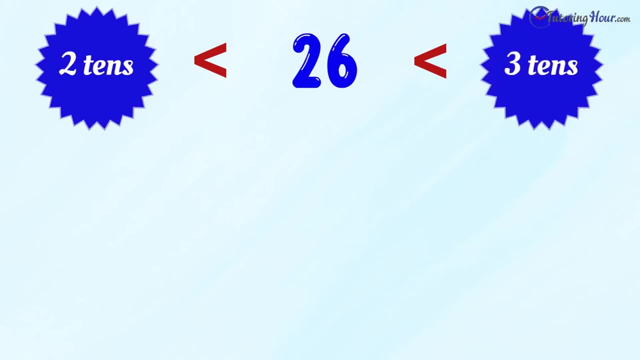 We have 2 in the tens place and 6 in the ones place. We know 26 is more than 2 tens but less than 3 tens. Therefore, 20 and 30 become our benchmarks. Now we need to decide if we will round down to 20 or round up to 30.. 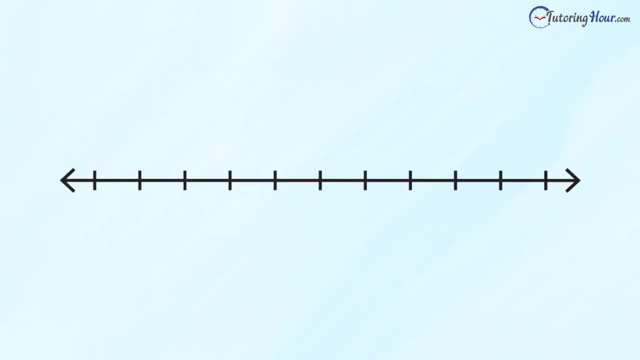 Let's put that on our number line, Starting off with 20 and going up to 30. We can see that 26 is between 20 and 30, but it is much closer to 30.. Let's animate our number line and make it look like a little number hill. 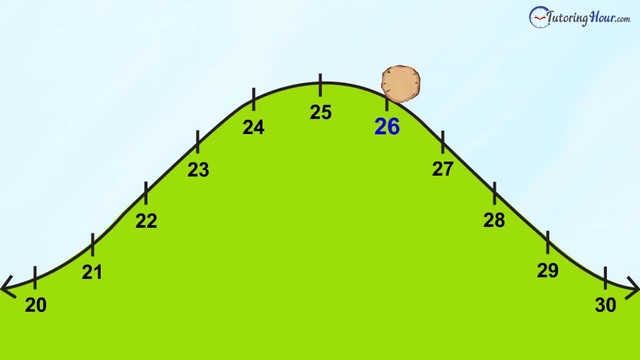 And imagine a log dropped off at 26.. Which side will it roll off? Obviously to 30. Now that implies we need to round up. But what if the log was dropped at 22? 22 is closer to 20.. It is clear that the log will roll back to 20.. 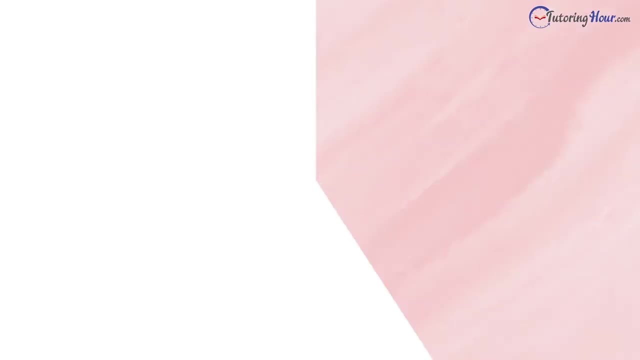 So here we are rounding down. That was fun, But is there a way to round off without a number line? Yes, There's a pretty simple rule to round off numbers. Let's try rounding the number 154 to the nearest 10.. 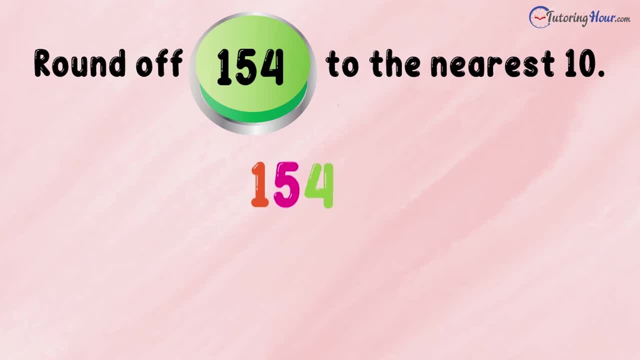 First we need to figure out the digit we are going to round off, the number to Which is the tens place? in this case, We have the number 5 there. With that done, we'll shift our focus to the digit that is on its right. 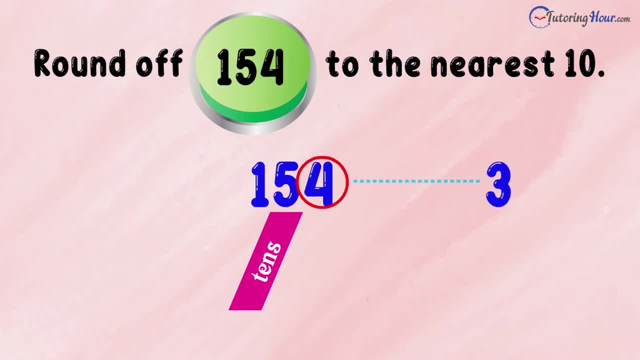 If you see a 0,, 1,, 2,, 3 or 4, then keep the targeted digit unchanged And drop the digits on the right of the targeted digit to 0.. That is rounding down 154, rounds down to 150. 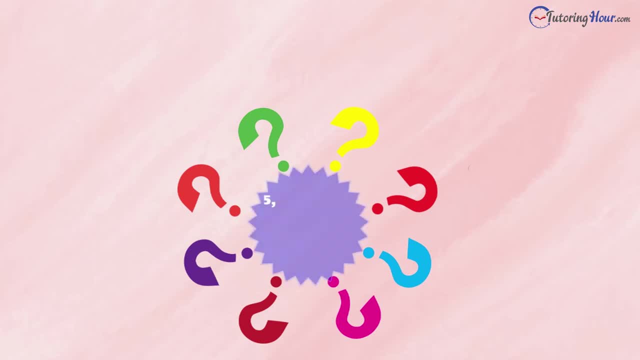 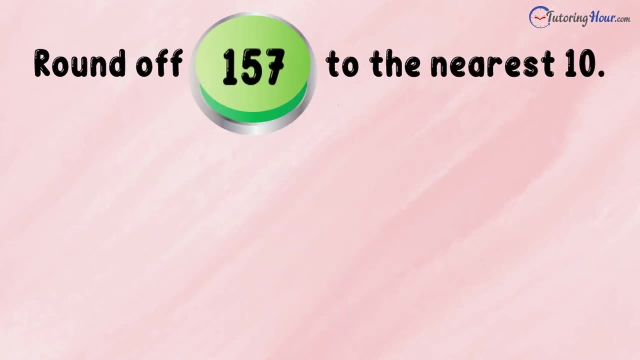 But you may ask what if we see a 5,, 6,, 7,, 8 or 9 to the right of the targeted digit, As in 157.. Then we need to add a 1 to the targeted digit, So we have 5 plus 1, making it 6.. 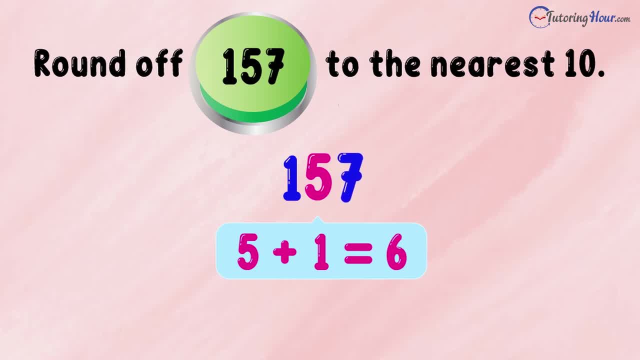 And change the digit to the right of the targeted digit to 0.. This is rounding up. The number 157 is rounded up to 160.. That's a pretty cool rule. Now let's move on to rounding the number 895 to the nearest 10.. 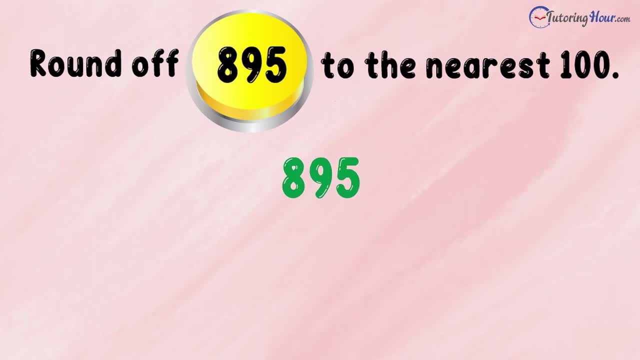 Our targeted digit in the hundreds place is 8.. So are we going to round up or round down Any guesses? Let's look at the number to the right of our targeted digit, The tens place. It has a 9.. So it is pretty clear we are going to round up to 900. 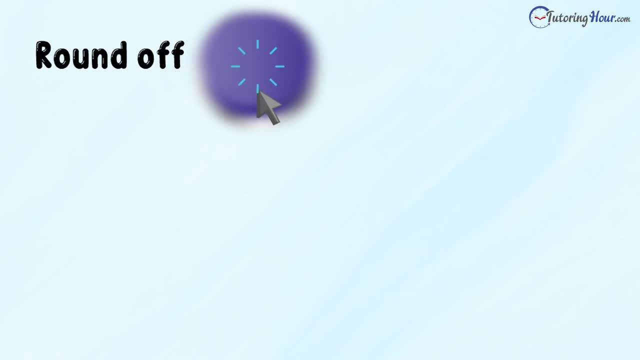 Let's upskill and try rounding off 4507 to the nearest 10.. The digit we are going to target here is 0. The number to its right is 7.. So 4507 rounds up to 4510.. That was quick. 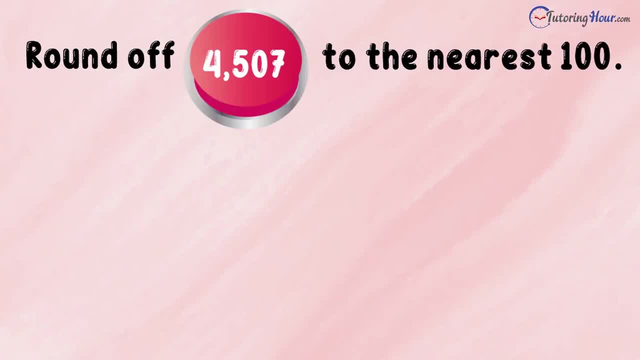 How about rounding the same number to the nearest 100?? Our targeted digit is now the number 5.. The digit in the hundreds place. We have the number 0 to its right in the tens place. It is pretty clear. we will round down the number. the hundreds place as it is. So 4507 rounds down to 4500.. Pretty straightforward stuff, this is. Let's move one more rung up the ladder and try rounding the same number to the closest 1000.. The targeted digit in the thousands place is 4.. 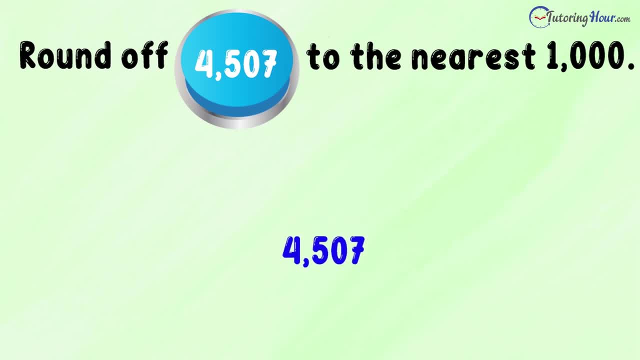 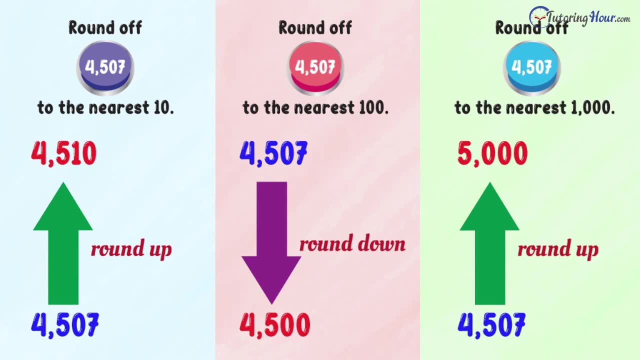 And the digit 5 to its right makes it apparent that we need to round up the number to 5000.. Looks like you are all set to round off and simplify numbers in your head and use this technique efficiently in and outside the classroom. Now it's your turn.